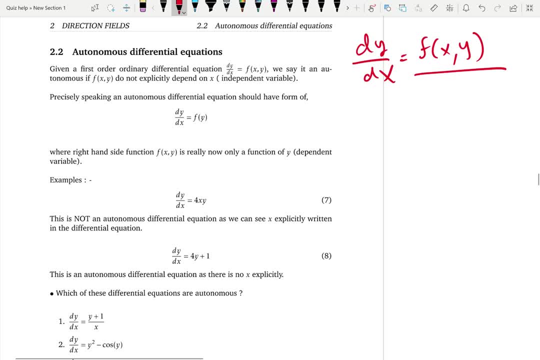 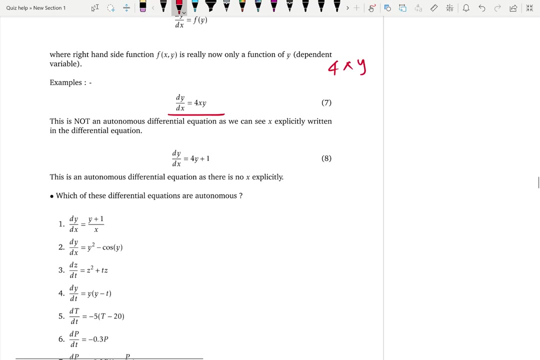 differential equation. So rather than writing f is as a function of both x and y, I would say it's function of just y, because you can only see the variable y or the dependent variable on the right hand side. Examples: dy over dx is equal to 4xy, So f is 4xy. Here you can clearly. 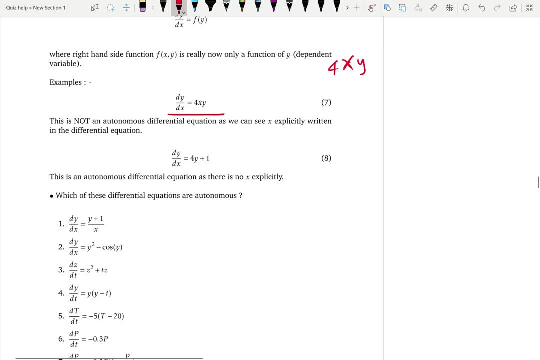 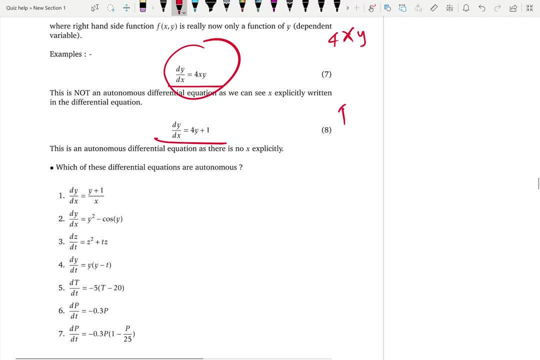 visibly see the independent variable x. So this is not an autonomous differential Equation but in differential, this differential equation, the right hand side is 4y plus 1.. You don't have x independent variable is right. So your right hand side only depends on dependent. 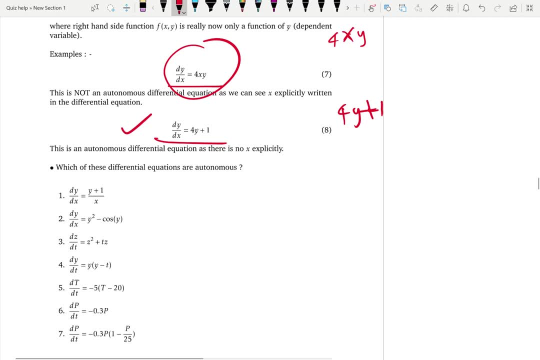 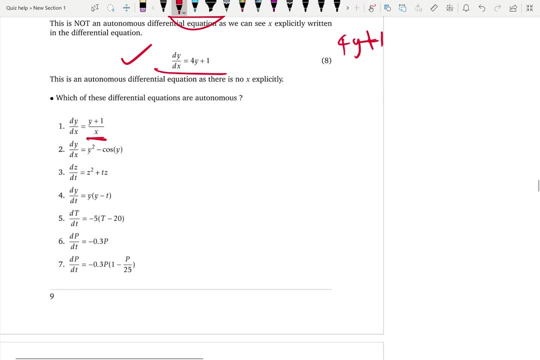 variable. So this is an autonomous differential equation. So let's do a quick exercise. Okay, all right, how about first one? Here you have x, the independent variable on the right, not autonomous Here, only y, right, only dependent variable. Autonomous Here. now, what is the dependent variable z? What is the independent variable t? 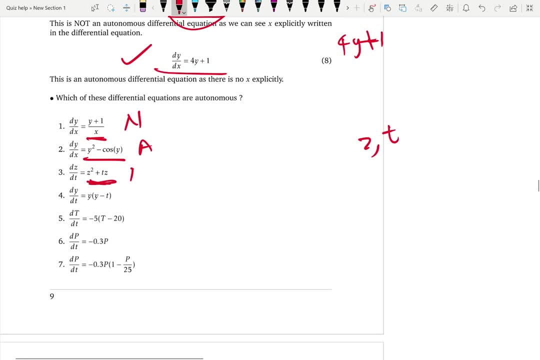 But you can see the independent variable on the right, So not autonomous. Here y is the dependent, t is the independent, But you can still see t in the right hand side, So not autonomous. Here capital t is the dependent variable. Simple t is the independent, which is not in the right. 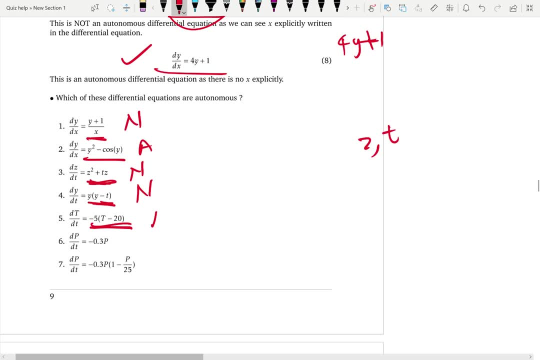 hand side You only have capital t, the dependent variable. So this is autonomous. Here capital P is the dependent variable and you don't see independent variable T on the right hand side. So this is an autonomous differential equation. Okay, All right. And then on the seventh one you can see the capital P is the dependent variable. Simple T is the independent variable. On the right hand side you don't see the independent variable, You only see dependent variable. So P is the. 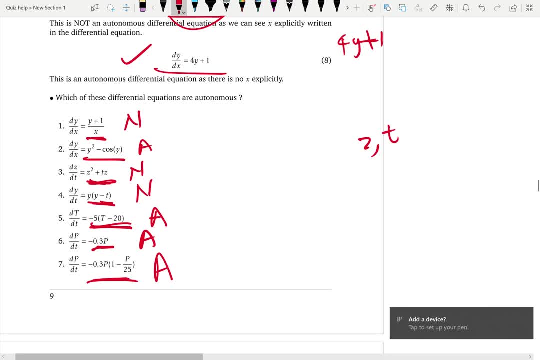 So this differential equation is autonomous differential equation because you can only see dependent variable on the right hand side. Okay, So that is an autonomous differential equation. We will discuss about them in future in more details. Okay, Thank you.